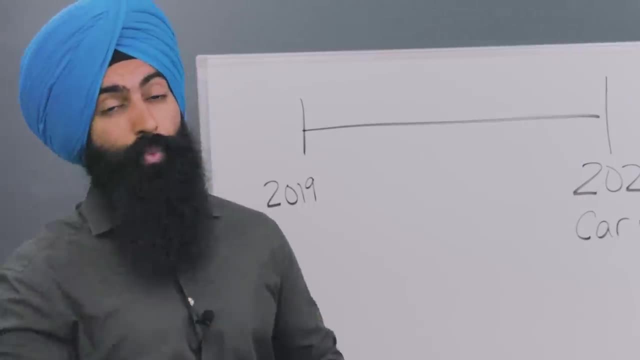 number one, how our economy changed and number two, how you can build wealth by systemizing your finances and building a system to number one: manage your money, but also start generating cash flow and build real wealth for yourself. So if you'd like to join me in this free virtual 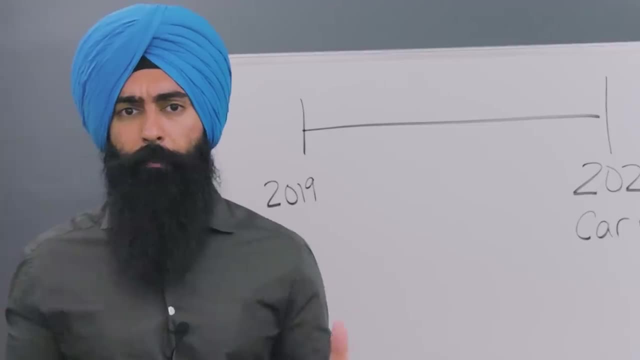 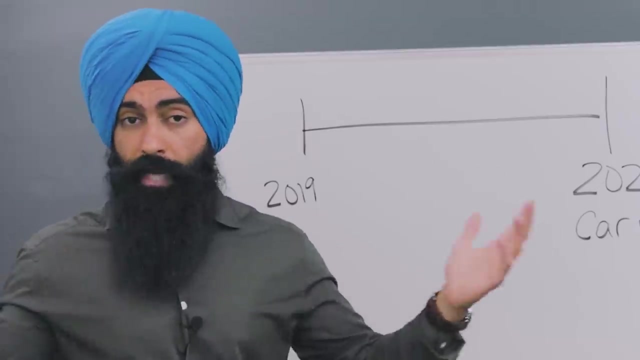 workshop. all you need to do is register, because there's a limited number of people that can actually join live. Every software has a limit to how many people can actually be there at the same time, So we have two times: one in the morning, one in the evening on February 6th. 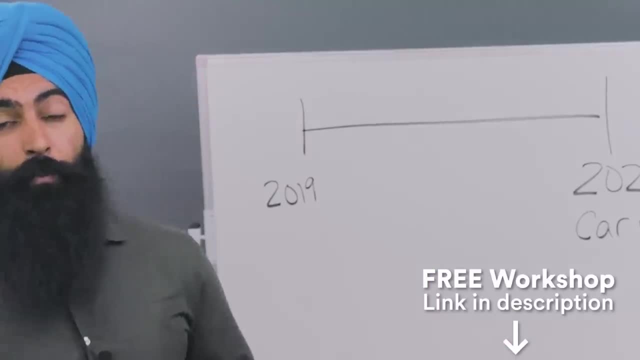 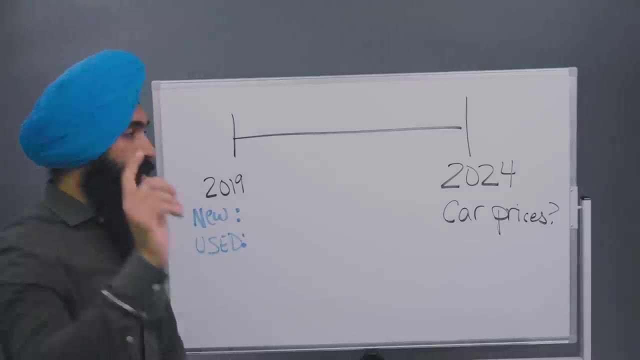 So if you'd like to join me, live for free. I got the link. You can join me on my first ever wealth building workshop down in the description below. Now back to the car market. In 2019, the average new car sold in America for just over $34,000, and the average used car in America sold for just over $20,000.. These numbers are a according to Kelly Blue Book. So, if we compare these car prices in 2019 to the car prices in 2023, because we don't really have much data in 2024, yet it's still January 2024 at the time- of recording this video, you'll see how much car prices changed in just a few years. In 2023,, the average new car was selling for just over $48,000, and the average used car was selling for just over $26,500 in 2023.. That means over the course of just ten years, the average used car sold in America for just over $34,000.. This means that we're already on the rise of the car market globally by about $26,500 in 2023.. That means, over the course of few years, new car prices jumped by around 41% and used car prices jumped by around 32%, While over that same time, between 2019 and 2023, wages grew by less than 15%. This is wages- people's incomes, Incomes- grew significantly slower than the prices of cars, which naturally can have you wondering, well, if people are spending so much more money for cars while incomes are not keeping. 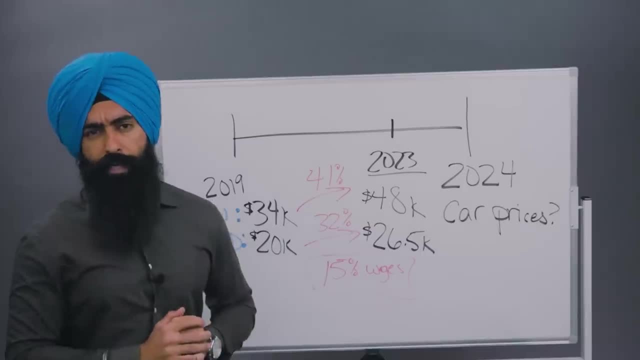 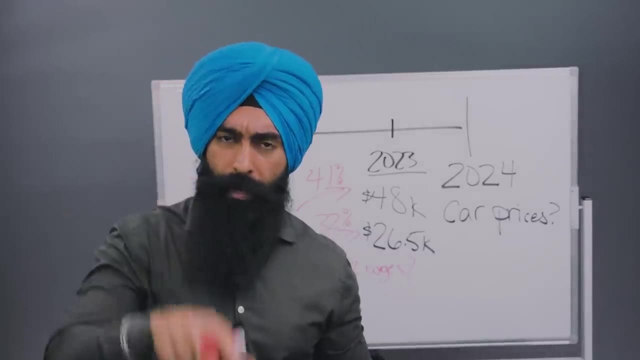 up. is that going to cause a problem? Well, hold on to that question for a second Now. personally, I am absolutely not an advocate for you to go out and finance a car, but I think it also helps to understand how car payments have changed over these years, because, well, unfortunately, most of America is financing their car And back in 2019, if you wanted to go out and finance this new car, you were paying around $554 a month. This was the average car payment in America in 2019, versus in 2023,, the average new car payment jumped up. to right around $726 a month for that same car. That means, over the course of these few years, your car payment also jumped by around 31%, while wages grew by less than half of that. In a normal economic environment, what you'd like to see is that car prices would be going. 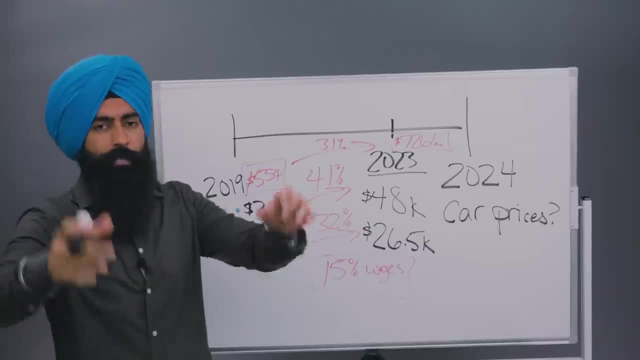 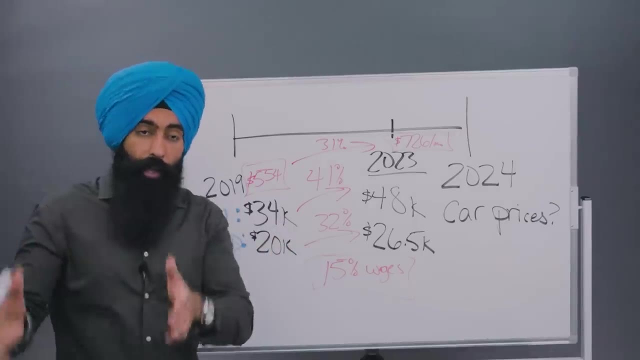 kind of relative to wages. Sometimes you see a little bit of discrepancy, but generally you'd like to see car prices growing along with wages. That means people are spending the same amount of the income relative to that car price. But that's not what we saw over. the last few years, We saw car prices shoot up much faster than wages, which is why, even though we saw car prices fall in 2023, people still feel like cars are extremely expensive, And to understand that, you have to understand what happened in 2020.. Oh, my numbers are really messed up To 2022. So let me clear off the whiteboard so we can understand what happened between these years. The number one main reason why we saw this huge skyrocketing of car prices between 2020 and 2022 was because we saw an imbalance between supply and demand between 2020 and 2022.. And let me start. 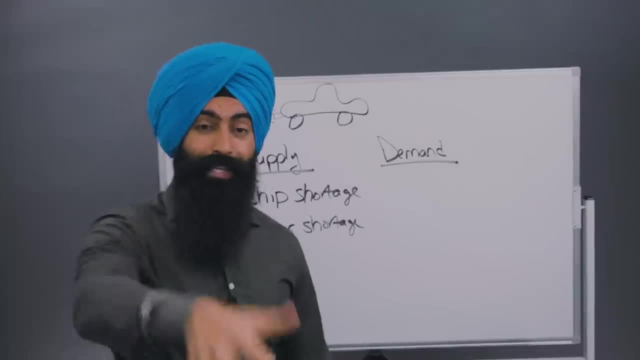 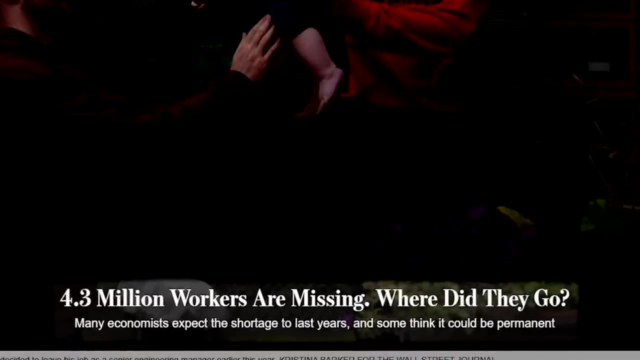 by talking about the supply imbalance that we saw Between 2020 and 2022, not only did we have a chip shortage, but we also had a labor shortage, making it very difficult for car companies to produce more supply, more inventory and more cars that they could sell. It feels almost like a 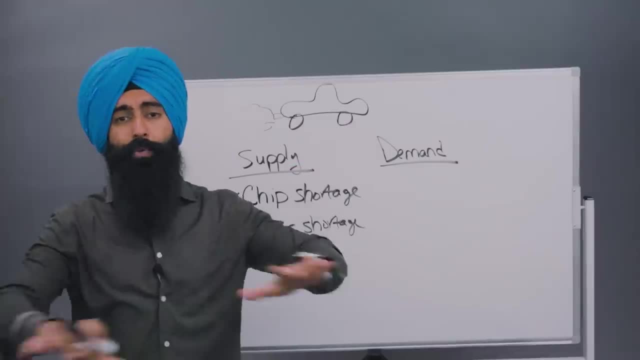 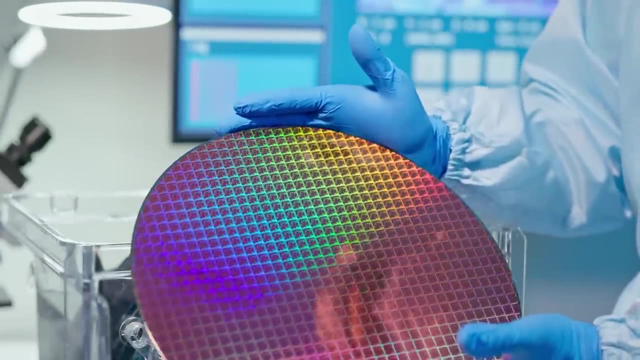 different world now, But in 2020,, when the pandemic hit, manufacturing across the world was shut down and our global supply chain was impacted heavily, which meant that car companies, who need these computer chips to build their cars, could not get a hold of these computer chips, which meant 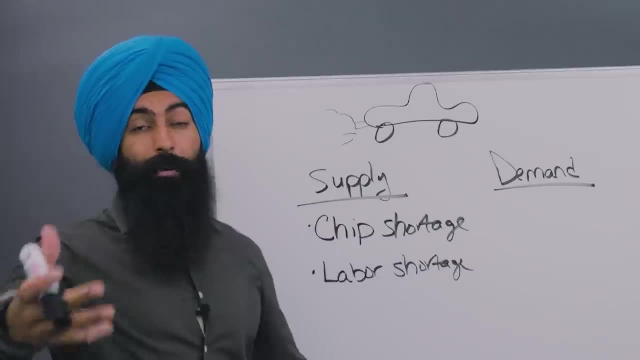 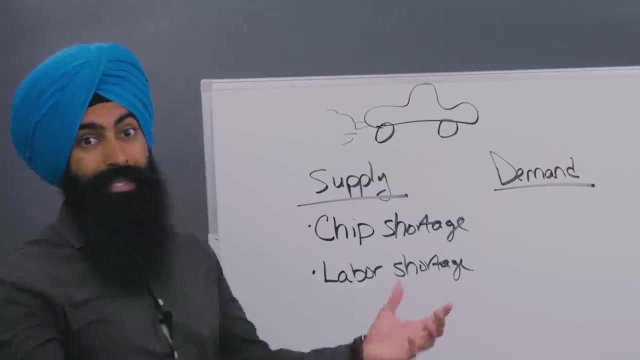 car companies could not produce more cars. So car companies couldn't get the products to produce more cars, which led to a lower inventory of cars being created. And then, second, when car companies did have the products to build cars, they couldn't find the labor to. actually build cars Because, if you remember, when 2020 and 2021 were going on, the government was giving out free money to people. There were big unemployment checks and people just didn't want to go to work. Some people were scared to go back to work because of the pandemic, So it was very hard for companies to go out and find labor. So number one companies couldn't get the parts. And then, even if they got the parts, they couldn't get people to actually put the parts together to build the cars, Because, even if you're not talking about the United States, you had factories. across the world that were shut down for way longer than the United States. So car companies were struggling to produce the products. So first they couldn't get products to build cars, They couldn't get the people to build the cars, which meant they couldn't create these cars to sell. 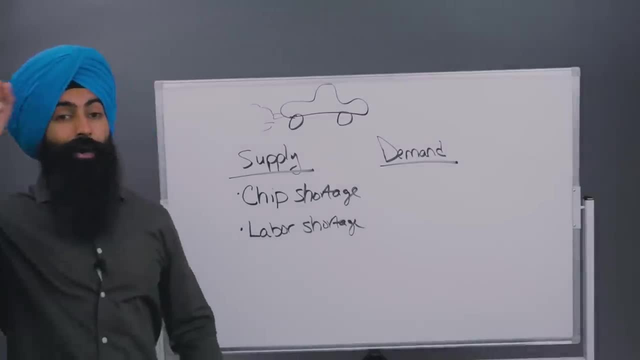 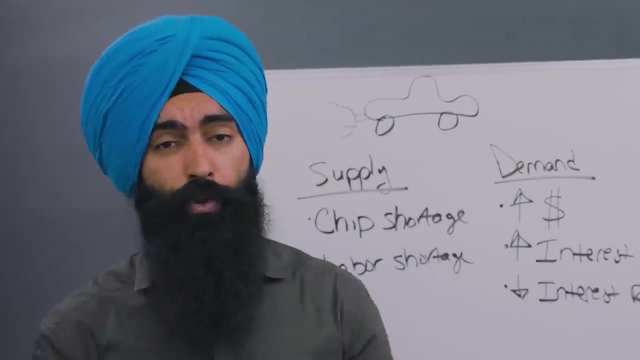 which then meant they have a limited amount of cars on the lot, while at the same time, everybody wanted to buy a new car. The car price boom started in 2020, but it really accelerated in 2021. And the reason for that was in 2020, in the early part of 2021,. people had very little expenses because you don't have to pay a mortgage, People weren't paying the rents, You don't have to pay a student loans And people were not going out to eat because everything was shut down. And on top of that, people were making more money through unemployment. checks, through stimulus checks, through whatever types of money they might be getting. Businesses were getting money from the government as well, So people were making more money. They had lower costs, So people had more money. Then, on top of that, you had this increased interest to go out. 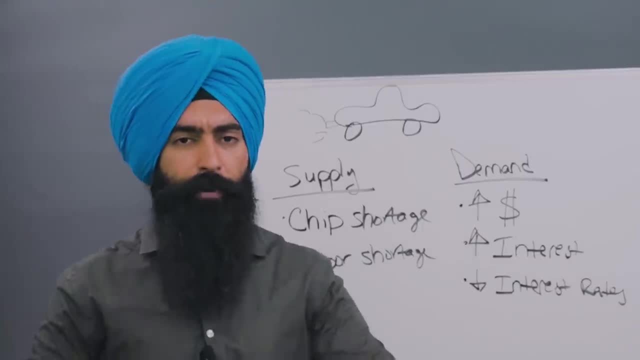 and buy a new car because of what people were doing, So people were making more money. They like to call this pent-up demand. Everybody had this pent-up demand because of the pandemic, not to mention the fact that Instagram really glorified. Everybody wanted to buy a G-Wagon. all those luxury cars in 2020 and 2021.. And then you also had some of the lowest interest rates ever, which meant that if you want to go out and buy a car, well, if you could find a car, you could get financing at some of the lowest rates ever. This created some of the biggest amounts of demand for car buying ever, while there were some of the lowest amounts of cars available for sale ever Now. I didn't do good in economics class. I almost failed my economics class in college. But what you learn in economics class is when you have. a low amount of supply and a high amount of demand. that generally causes the price of things to go up, And that's what we saw happen in the car market. You had everybody that wanted to buy a car, nobody who had cars available for sale, which meant that if you had a car available, for sale. you could then sell it to anybody for a big profit, In fact. I talk very openly about how cars are liabilities, how you're going to lose money with your car. Well, for a brief period between that 2021 and 2022 time- even a little bit into 2020, people were selling their cars at 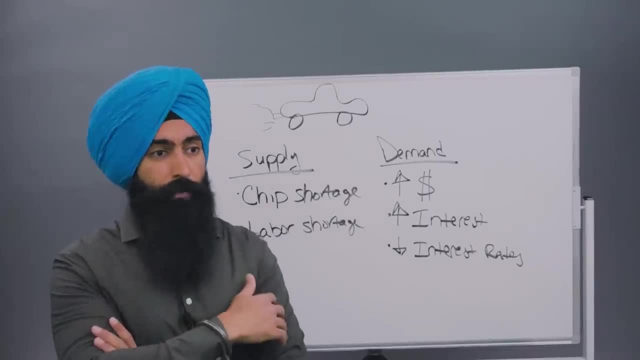 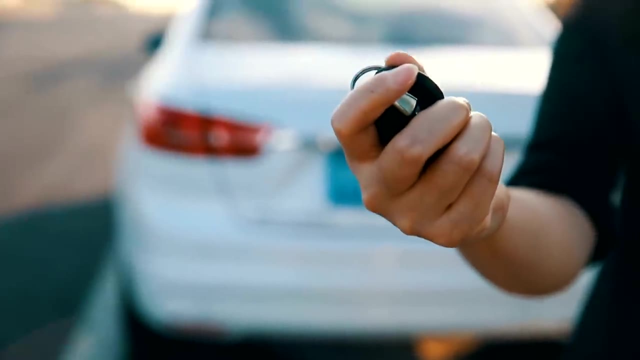 huge profits. You could buy a car, drive it around and just tax the car and then sell it for a five to ten thousand dollar profit after 12 to 18 months of driving it around. It was a very strange economy And the reason was you had such a low supply with so much demand that people wanted. to buy cars, especially nice cars, because people had money, they had the interest and then you had these low interest rates. So people were wanting to go out and buy these nice cars, which then caused car prices to boom, starting in 2020, especially in 2021 and then into 2022. But then things started to change in 2023. See in 2022,. that was when the Federal Reserve Bank started raising interest rates, But there was still a lot of other demand. People still had cash ready to pay for cars even if interest rates started rising, But the Federal Reserve Bank continued. raising interest rates through 2022 into 2023. And 2023 was when we started to see demand start to cool down And that's when the Federal Reserve Bank started to raise interest rates. And that's when we started to see demand start to cool down And we started to see supply start to pick back up. 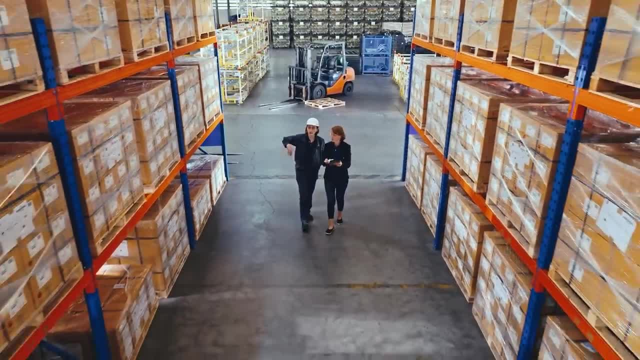 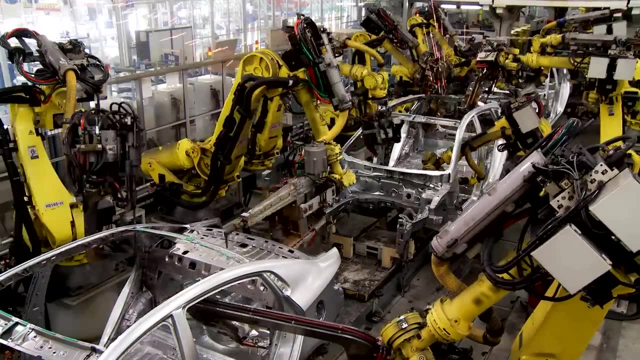 Why did supply start to pick back up? Because we started to see the supply chains ease. We started to see systems ease. We started to see the manufacturing plants open back up like normal, which meant now car companies were able to build more cars- kind of like normal again. And then, at the same time, demand started to fall. Now, there was still high demand, but it started to fall relative to the crazy demands that we saw in 2021, because then people started to realize, oh, I can't blow my entire 401k on a car. People realized, yeah, I might. 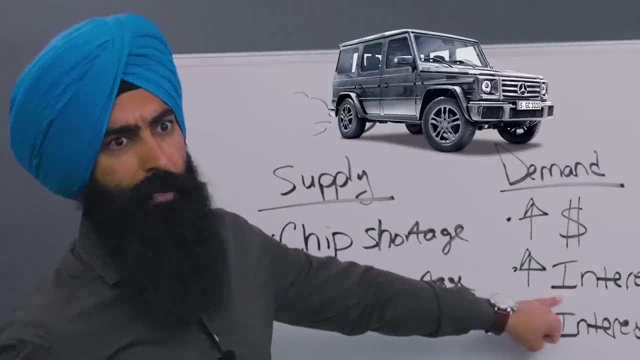 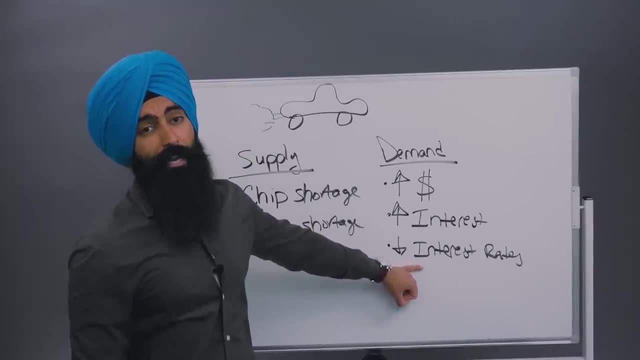 like a G-Wagon, but maybe I should start investing for retirement, Or maybe I should care about my credit card debt instead of a G-Wagon. And then interest rates were a whole lot higher in 2023, because the Federal Reserve Bank raised interest rates 11 times between 2022 and 2023.. This lower. demand, and now this higher supply then caused car prices to finally start falling in 2023. And it wasn't just new cars: Used car prices fell by around 20% between the 2021 peak and 2023.. So mathematically today, if we ignore, interest rates, assuming you're not going to finance a car. the dollar amount that you have to pay for a car today- assuming you're going to negotiate the price- can be less today than what it was 12 months ago or 18 months ago, which is good news if you want to go out to buy a car. because that means you can get a cheaper car today than a year ago. But the reason why car prices still seem so much more expensive is because, well, number one, if you're financing your car, you're paying higher interest rates today than you were in 2022.. And then number two, the reason why it feels so expensive is because car prices have grown so much between 2019 and now. So even if car prices fall by 10%, they still seem expensive if you compare car prices to what you thought they were before the pandemic. What we do know for a fact is that car dealerships are starting to feel the impacts of higher interest rates, And if interest rates stay higher for longer, that's going to put more pressure on car dealerships and car companies to lower the prices of their cars. How do we know? Well, you can just take a look at what's happened with some of the startup companies, especially in the car resale market. We all might remember what happened with Carvana back in 2022. Where Carvana was on the verge of bankruptcy because, well, they just weren't selling as many cars as they thought they would have. And if you look even more recently, there was a very hot 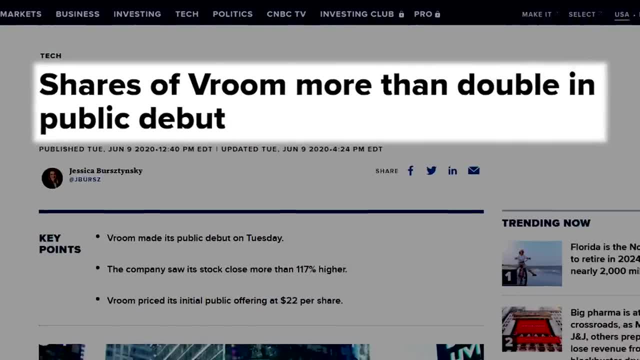 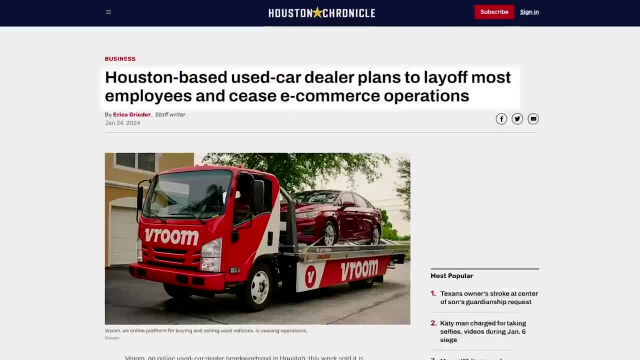 car resale startup called Vroom, which had a very hot IPO in 2020, which then, in 2024, January 2024, decided that they're going to shut down their used car selling division And they're going to lay off. 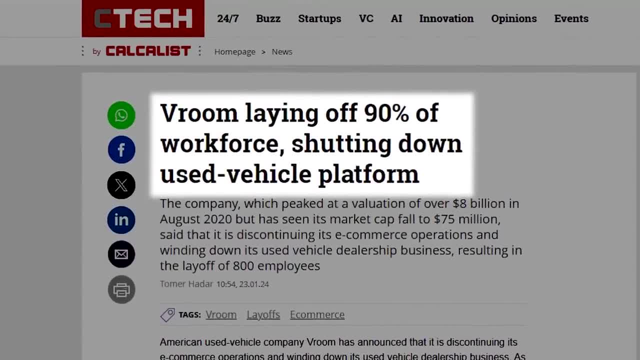 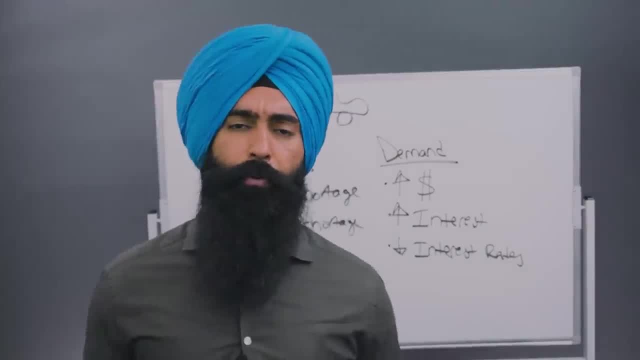 pretty much every one of their employees, because they don't have the same demand of people buying these cars And with the high interest rates, it's very hard for them to make any money, And not to the fact that we've been seeing the used car prices for G-wagons and other luxury cars begin to fall. Actually, they've been falling for a little while now, And this is partially due to the fact because people were way overpaying for these cars, like G-wagons back in 2020 and 2021, where people were paying $10,000 to $20,000 over MSRP standard, And now they're letting go of these cars for a huge. 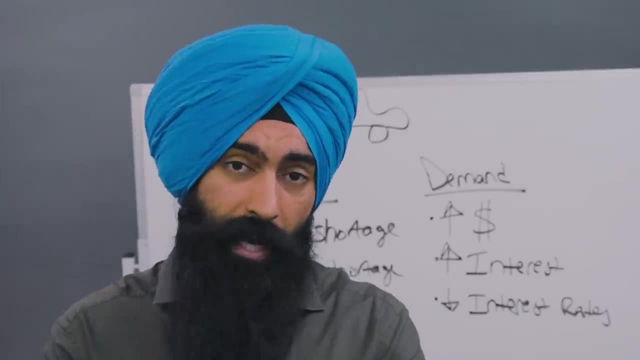 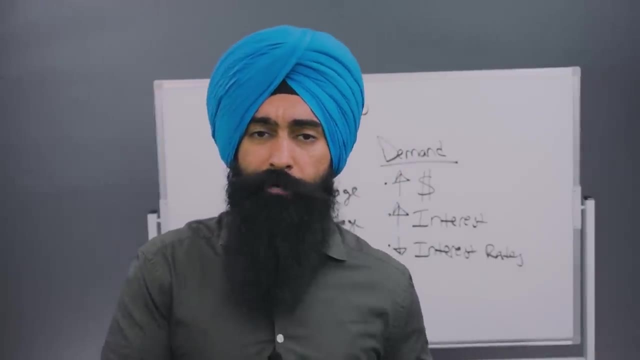 discount because, well, you have a lot of people selling these G-wagons at the same time. So now for those of you who are in the car market, what does all this mean? Number one: I don't really care what's going on with interest rates when it comes to loans for cars, because I have no interest. 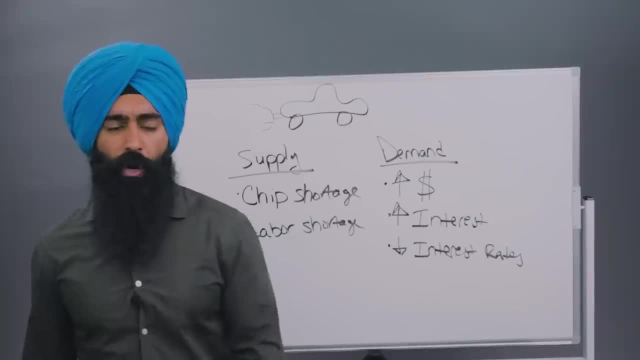 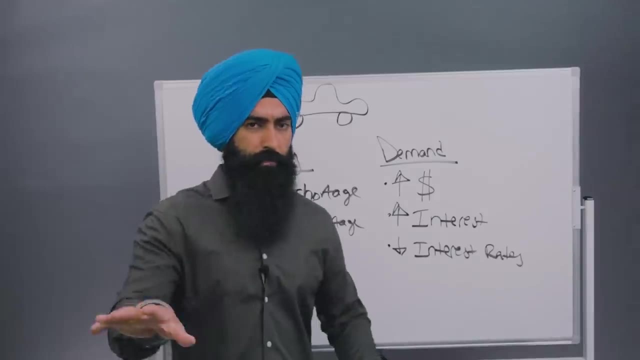 in financing a car, And I don't recommend anybody finance a car, because when you're financing a car you're paying interest on a car that's losing value, which means it's like a double whammy: The car is losing value and then you're paying interest on the car that's losing value. But interest rates are something that you have to pay attention to, because they impact here the demand side of cars. See, what we know is that supply and demand impact the price of cars, And we know that supply has come up in 2023.. 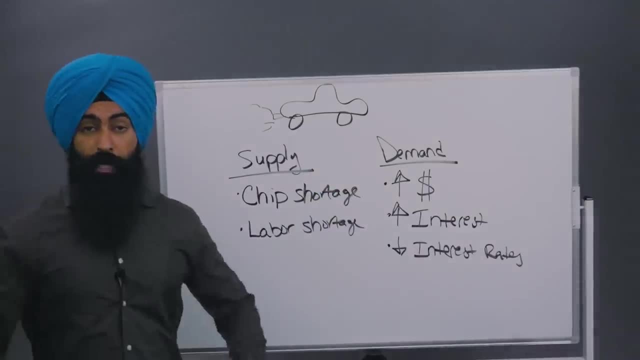 This is because the chip shortage has gotten fixed and this labor shortage is much better. So car companies are producing cars much better today than what they were two years ago. Is it perfect? No, but it's much better today than what it was. So we know that the supply of cars has